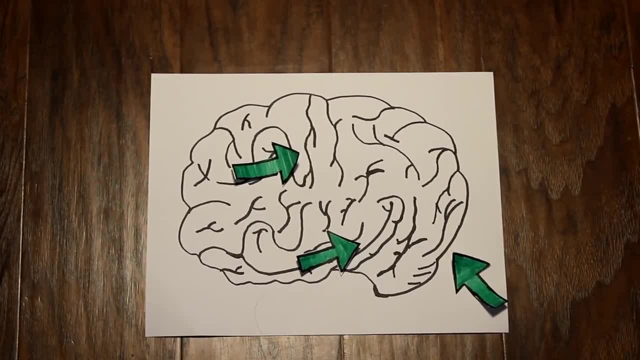 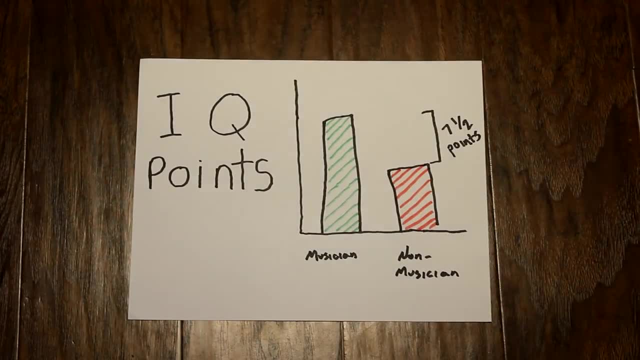 could do to improve the mental capabilities of a struggling student. It is shown that, on average, a recipient of music education's IQ is 7.5 points higher than someone not studying music. It is vital that music education should be supported and possible for all to become a music teacher. We're all learning to study music, but we need to learn how to use the imagination or means to do so. So I'm changing the controls of our brain. We need to learn to be a prodigy or genius to experience the benefits of music education. 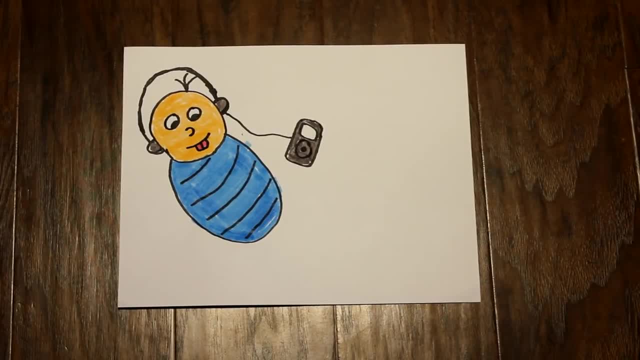 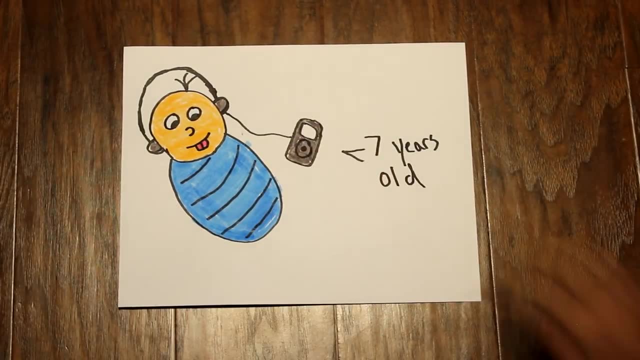 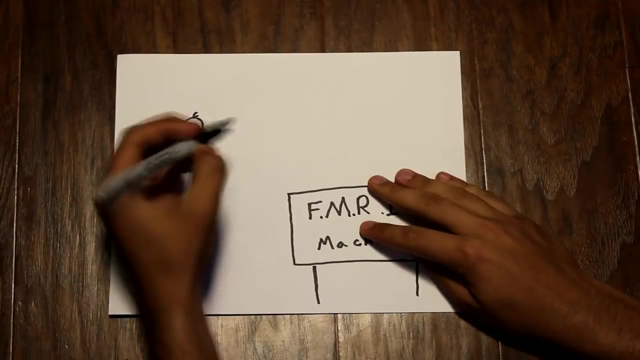 music education becomes an essential part of the academic curriculum at a young age. Most neuroscientists believe that for maximum benefit, a child should be introduced to musical training before the age of seven years old. Music quite literally shapes the way that we learn. An experiment was done where 18 babies between one to three days old were placed inside of an 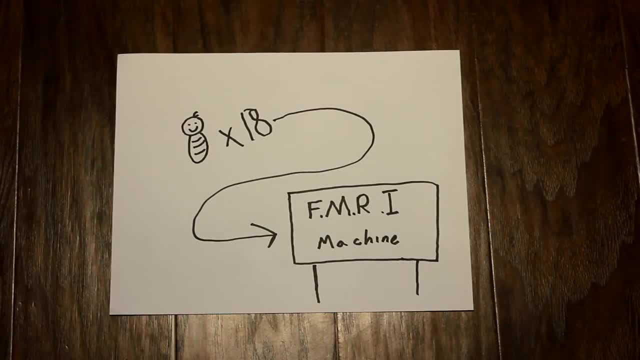 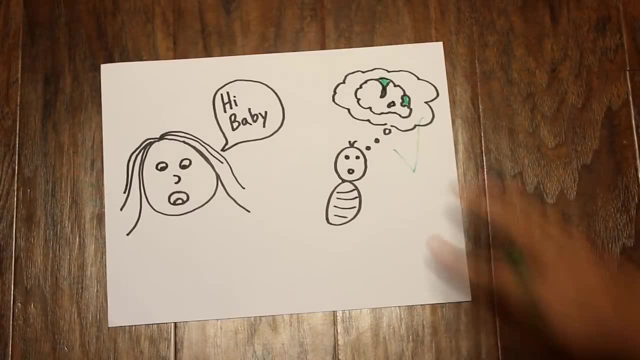 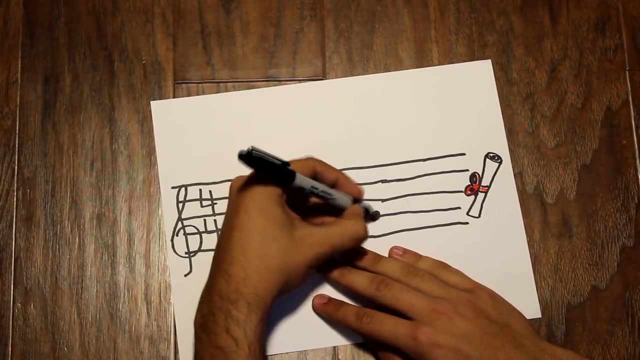 fMRI machine in order to examine their brain activity while being subjected to different types of stimulation, While listening to their mother's voice. the scan showed that all areas that the brain used, the musical training, were being used by the baby to understand their voices. We use music to understand language, tone, cadence and emotion. we are innately musical, being so. 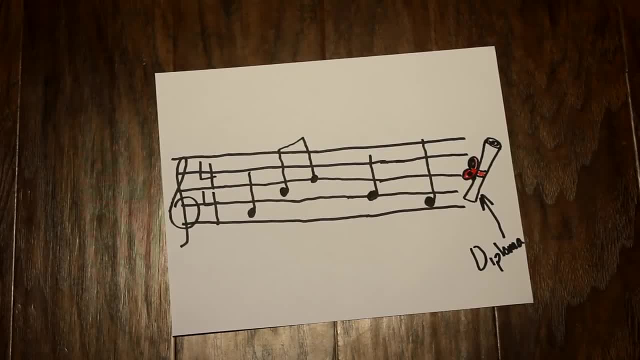 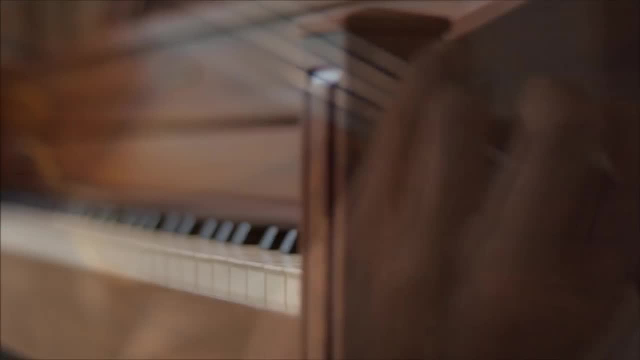 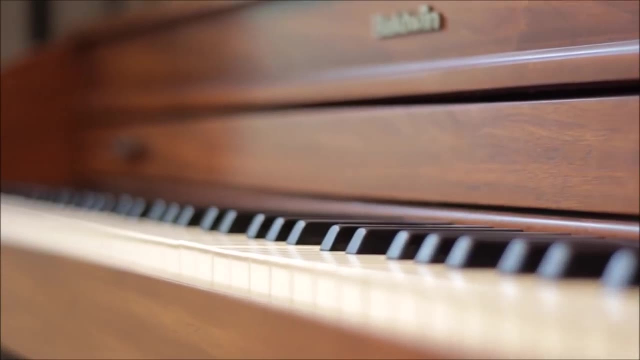 encouraging that growth can only make us better people and scholars. Music is not just an art, it's an idea. You hear a melody and it moves you, makes you feel emotions. The notes and rhythms imply things, but it's up to the listener to give that meaning. 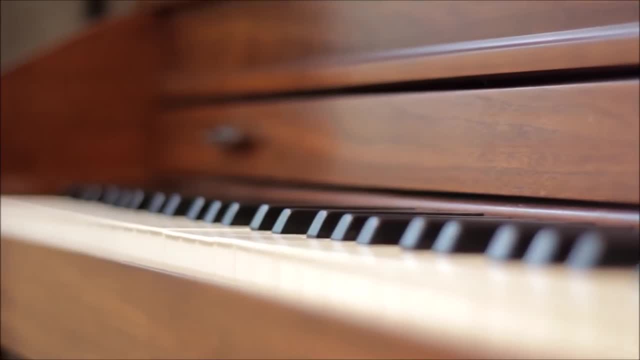 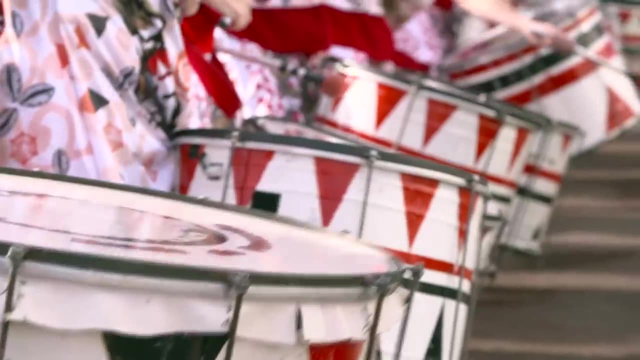 Music is abstract, It's 디자inational. it's abstract, it's objectглядical- it's abstract. It doesn't need anything outside of itself to be understood. Music empowers people to create and experience things that they would have no means of experiencing otherwise. 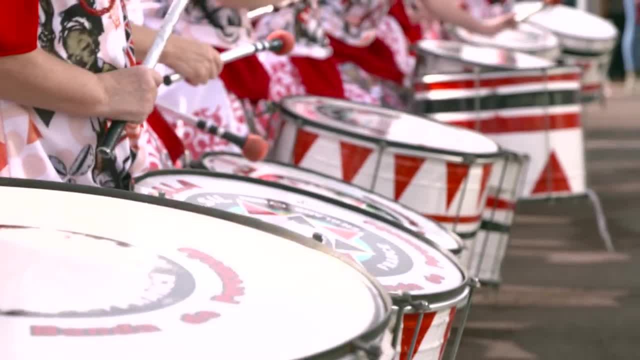 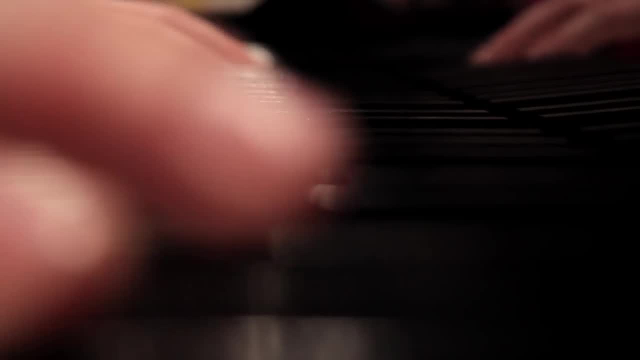 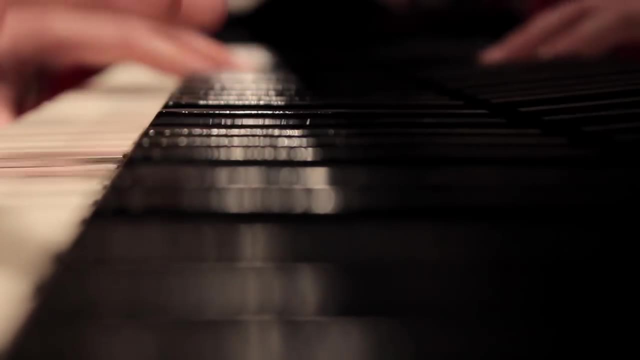 Music can build you up or tear you down. It is a powerful force that needs to be understood. It stands tall on its own and deserves to be taught for that reason alone. It encourages discomfort as you try something new. It encourages critical thinking as you analyze its infinite possibilities. 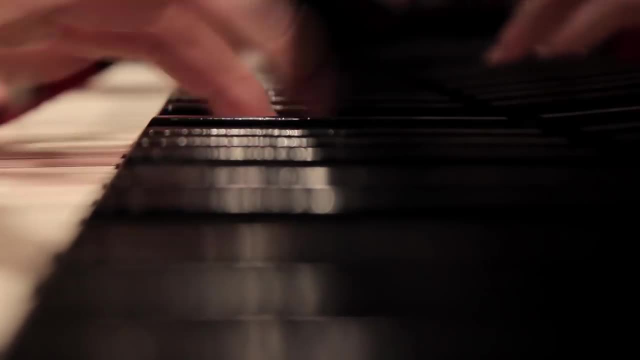 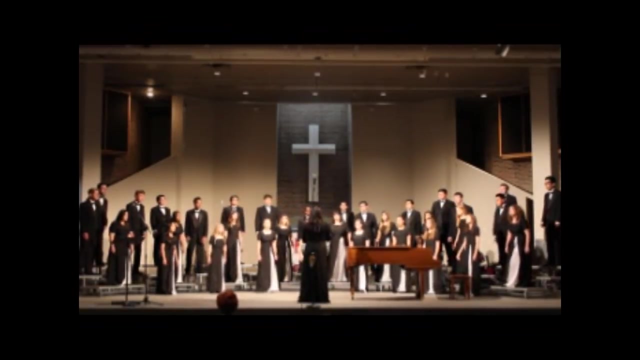 It encourages creativity as you work to interpret a beautiful piece of music, And it encourages self-discipline and personal growth as you work to better your talents. Imagine a world where music education is another part of the daily curriculum. All students head to piano class after algebra. 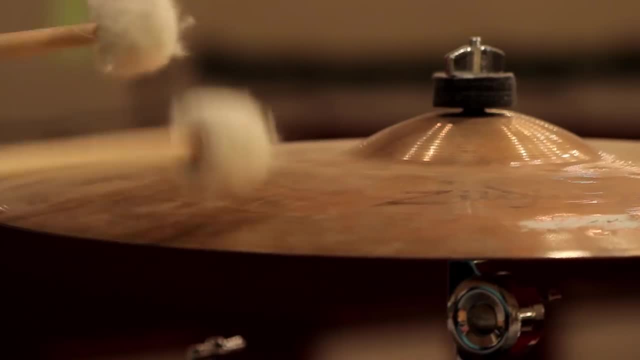 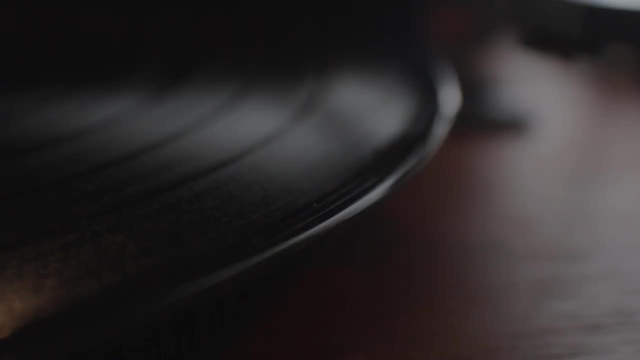 or choir rehearsal after lunch. A more well-rounded student body produces higher test scores or even a higher graduation rate. In a lot of ways we can predict its benefits, but in a lot of ways we can't. So I encourage you to ask yourself.